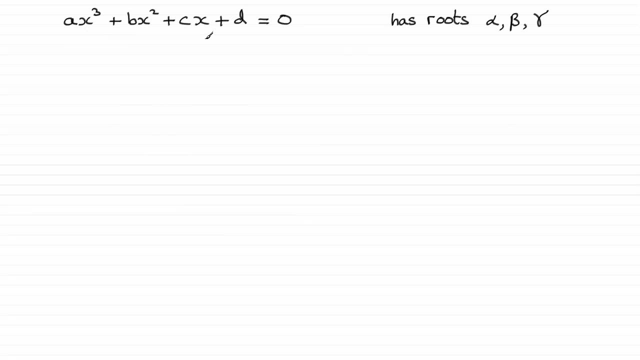 one here: ax cubed plus bx squared, plus cx plus d, equals 0.. Let's say it has roots alpha, beta and gamma. That means x would equal alpha, x equal beta, x equal gamma. Then clearly, if I was to factorize this equation it would have taken. 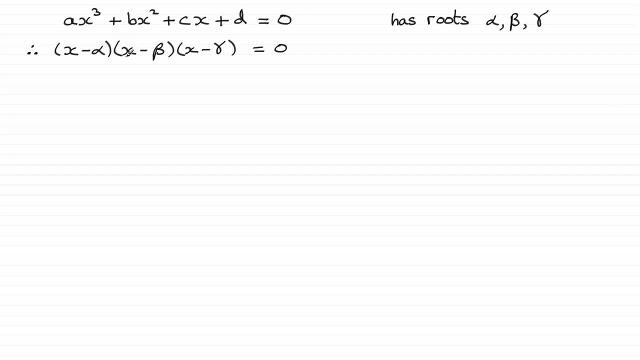 on this kind of format, leading to each of these factors equaling 0, meaning x equals alpha, x equals beta, x equals gamma. Now if I expand the last two brackets here in the usual way, then we'll see that x equals alpha, x equals beta, x equals gamma. 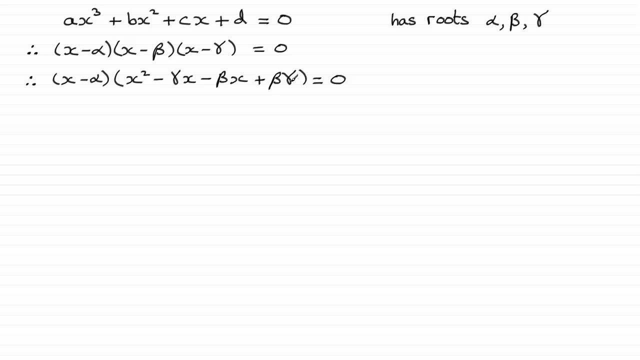 What I'm going to get is something like this: And then if I expand through with this first bracket, x times all of these terms, followed with minus alpha times, all of these terms, then I'm going to get this line here. And if I simplify this, group up the terms and factorize, 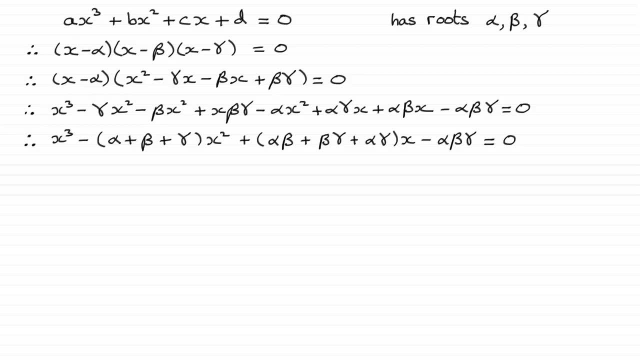 I'll get a line like this: Now, if I label this equation 1c and I divide through by a, then what we're going to get is this equation here: x cubed plus b over a times x squared plus c over a times x plus d over a equals 0.. 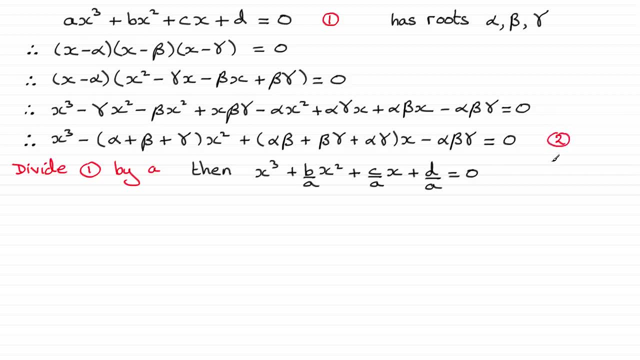 Now suppose I label this equation here 2 and this one equation 3.. Now what I can do now between these two equations is compare the coefficients. So if we compare the coefficients between equations 2 and 3, then let's say we look at: 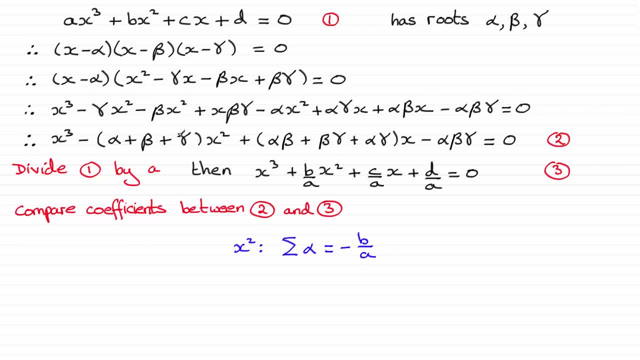 comparing the x squared coefficients, You can see that the sum of the roots alpha plus beta plus gamma must be equivalent to minus b. over a Notice, we've got a negative here and a plus here, So I've just switched across the two signs And I've written this for short as: 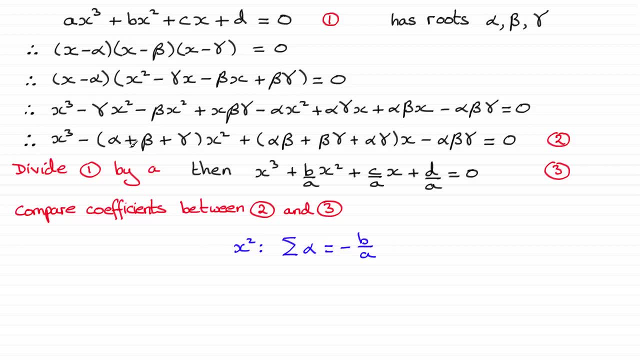 the sum of the roots as sigma alpha. That would be alpha plus beta plus gamma. if I was to expand it out Now, if we look at the coefficients of x, you'll notice that I've got here the sum of the products of pairs of roots And that must be equivalent to c over a.